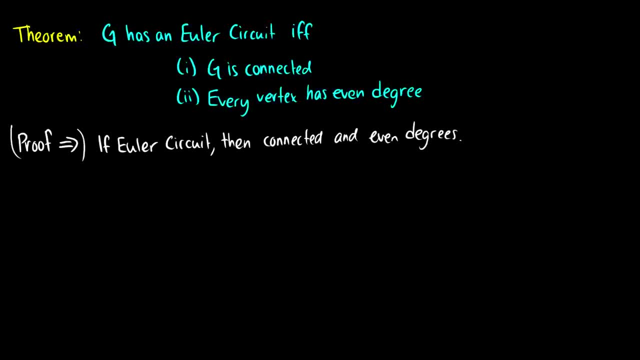 has an Euler circuit if two conditions: G is connected and the second condition: every vertex has an even degree. So let's say, if Euler circuit then connected, an even degree. So let's say here: so there's an Euler circuit, the graph definitely has one. So clearly the graph has to be connected. 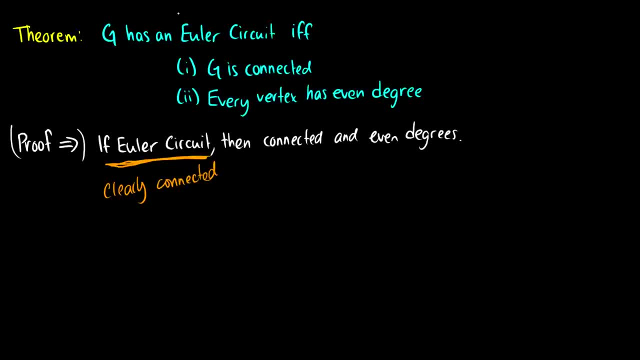 And I'm going to show you an example. and you can do this in words and you're proof. I'm not going to write out word for word, I'm just going to kind of show you with pictures what's going on here. So suppose Let's take a very simple, simple Euler circuit. 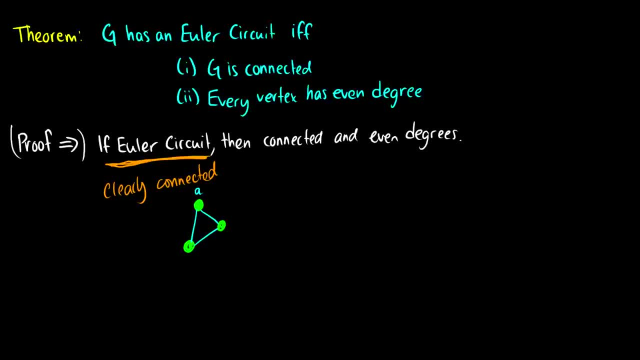 So we see here that we can go from A to A and use every edge exactly once. That's pretty straightforward. We just go down, up and back up. But if we have a disconnected graph, so let's say we have a portion. 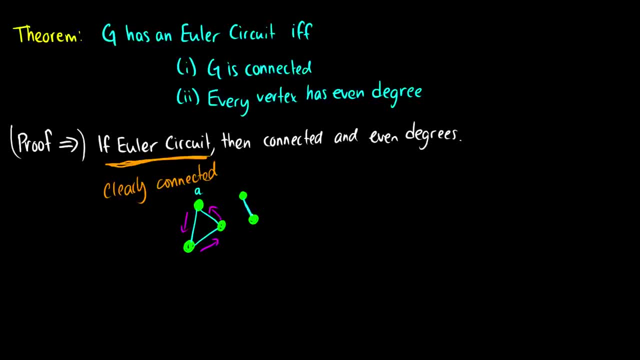 over here with this edge. well, it's impossible to get over to that edge to use it So clearly. it can't have an Euler circuit if it's disconnected. So if there is an Euler circuit, we know the graph is going to be connected. 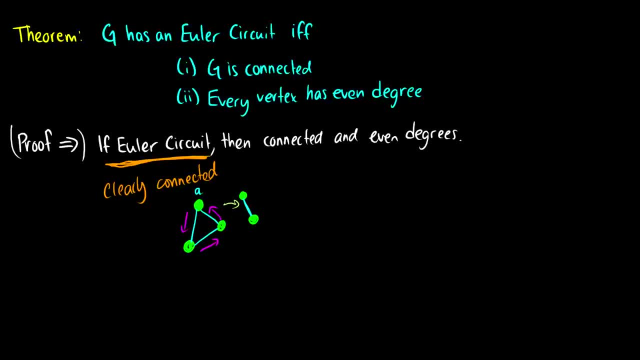 It has. each and every vertex has an even degree. So what's that mean? Well, let's take a look. Let's call this our Part 1 over here, And then Part 2 here. Let's take a look at a graph with an odd degree. 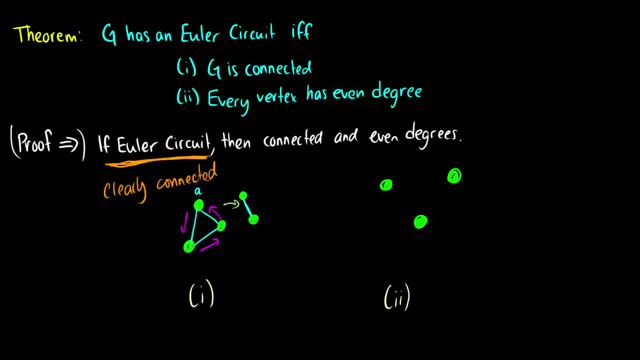 where one vertex has sorry, there are two vertices that have an odd degree. So let's do- Actually I know what we'll do- We're going to give this one two edges. we're going to give this one one edge. So we want to go from A back to A. So here's what happens if 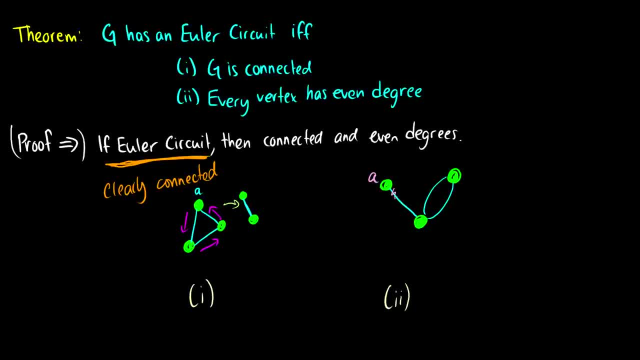 we have a vertex of odd degree. We leave, Okay, we leave A, And now we can't ever return, Ever. So we can't have an Euler circuit. So if the graph has an Euler circuit, then clearly G has to be. 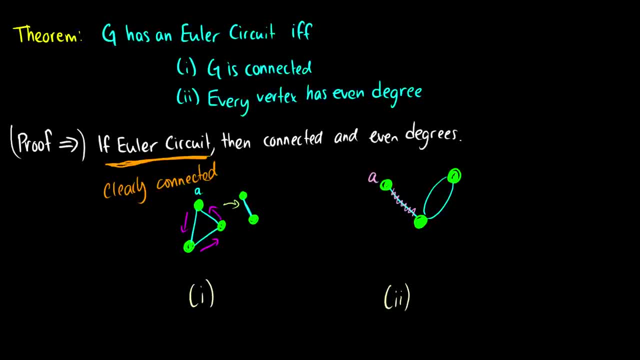 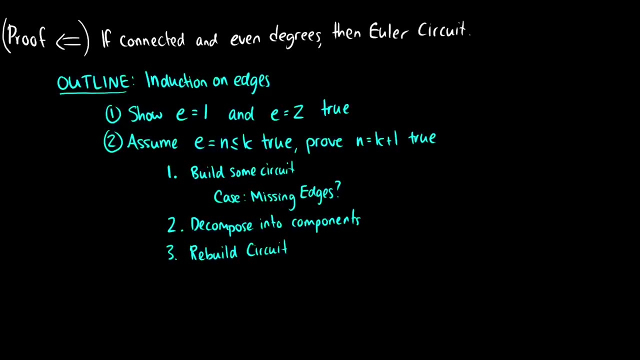 connected And every vertex must have even degree, because we have to leave and return. So if there is an Euler circuit, we know for sure that it's connected and it has even degree. So let's prove the other way, which is a lot harder. I'm going to outline the proof in words and then we'll go. 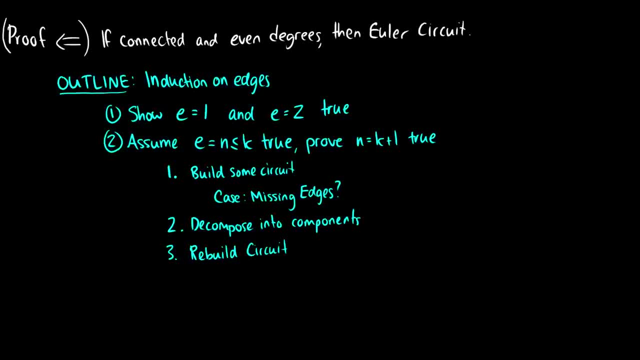 through it. So we're going to do an inductive proof on edges. So we're going to show that if there's one edge and two edges, then we're going to have an Euler circuit. And if there's one edge and two edges, then we're going to have an Euler circuit. And if there's one edge and two edges, 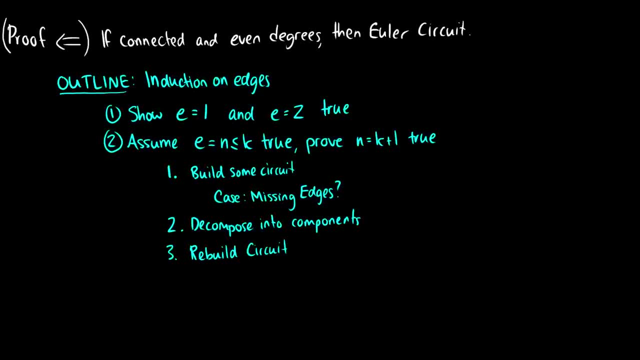 where the graph is connected and has even degree, then we can construct an Euler circuit. Then what we're going to do is just assume that some graph has K edges And then we're going to add an edge And we're going to see if we can reconstruct an Euler circuit from it. So we're 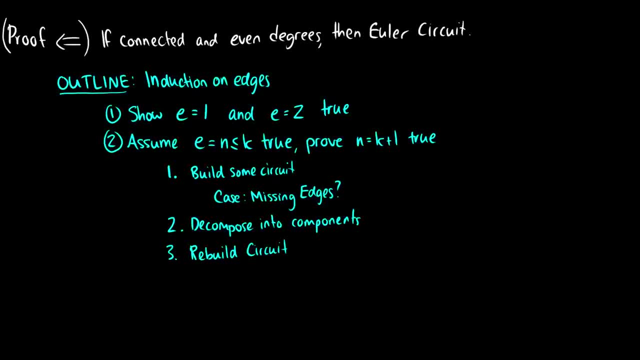 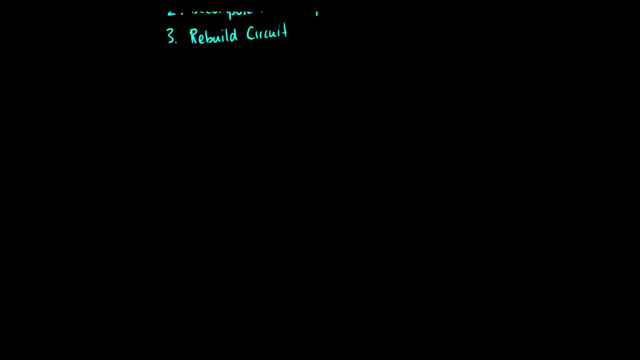 going to build a circuit, We're going to decompose into some smaller circuits And then we're going to rebuild it and show that we have an Euler circuit. So let's do the base case. We have to show that when the edges are equal to one edge, or two edges, it's true. So let's let E. 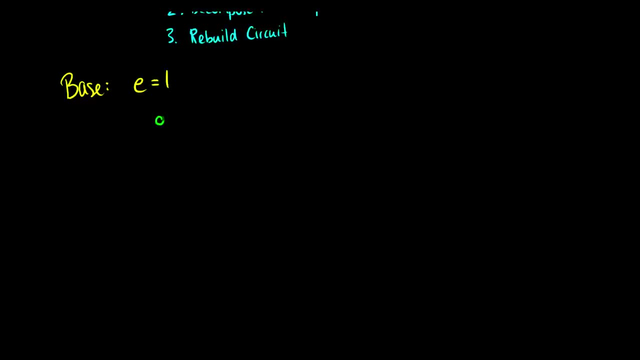 equal one. So if there's one edge, then well, we're going to have to have a loop. So there's a loop, So we can go all the way around And that's an Euler circuit, Okay. And if we have two edges, so remember. 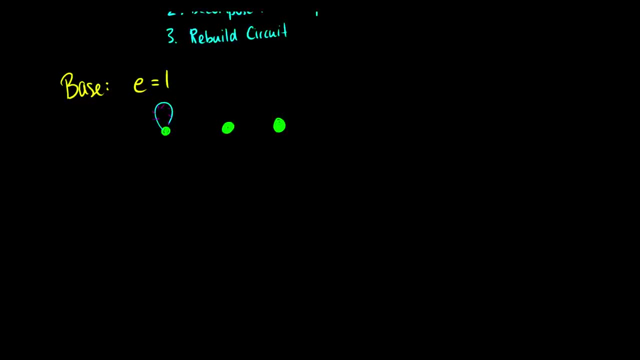 here edges has to be one because- or sorry- the number of vertices has to be one, because it's connected And every vertex has even degree. So those are the conditions that we're saying: okay, it is connected, it does have even degree. So this is the only way to. 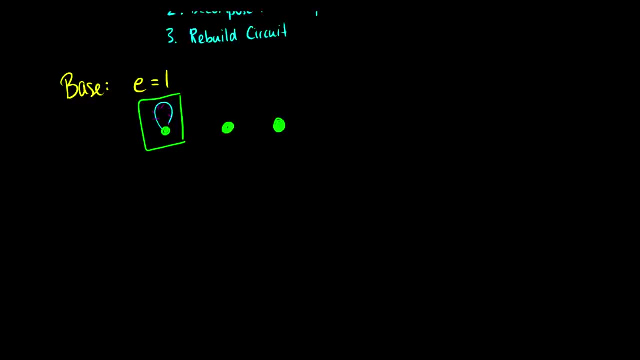 we can make it connected and even with one edge. Okay, so here's edges equal two, So we want E equal to two. Well, there's actually two cases here. One case is we have two loops, So I'm going to actually do this like this. Well, clearly there's an Euler circuit, because we can go on. 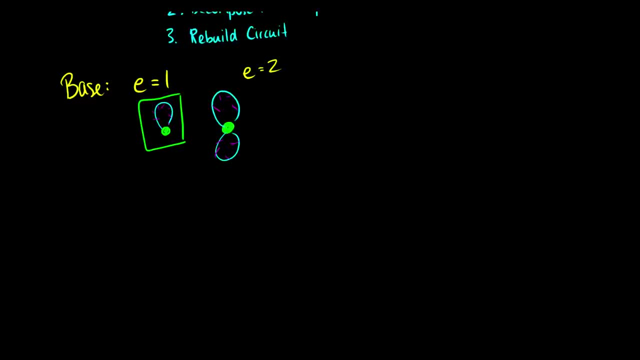 this edge, then on this edge, in any order. But another case is when we have actually we can do this here- Yeah, I think we can. So we can do this sort of graph, So we can go from A to B and then we can go from B back to A. So those are the only two graphs we can do where 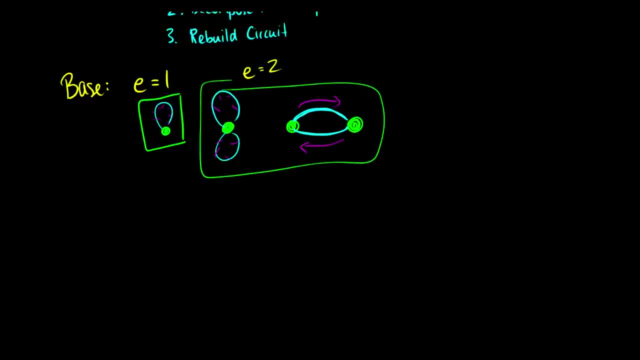 the edges are two, where again the graphs have to be connected and each vertex has to have even degree. So that's the base case. Now for the induction hypothesis. we're going to assume that n less than k edges are equal to one. So we're going to assume that n less than k edges. 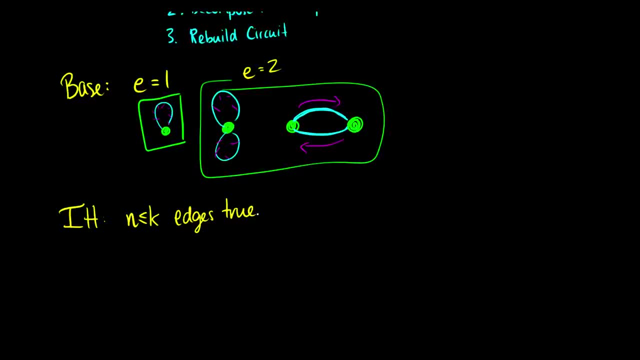 are true. So this is a strong induction. So we're not just saying that when it has k edges, it's true. We're saying that if it has any number less than or equal to k, it's true. So this is strong, And we want to show that the edges equal to k plus one has a circuit. So here's what we're. 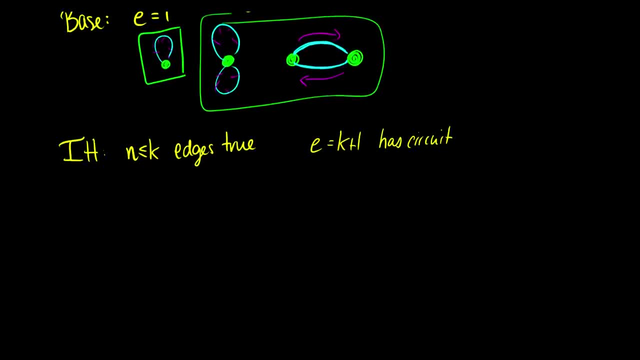 going to do? We're going to take a graph. We're just going to call it graph G And we're going to say it has k edges. So we don't know what it looks like, But we're going to start looking at. 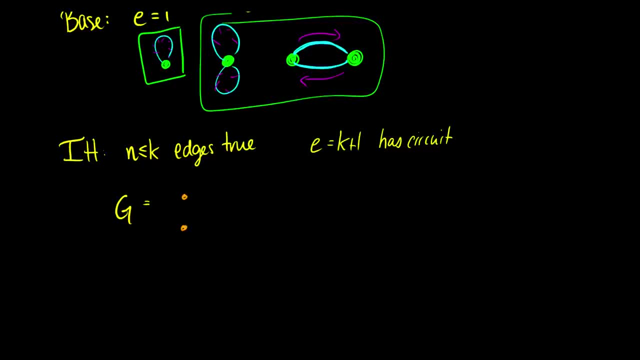 the edges here. So it's some graph. Let's take this graph, for instance. Okay, this has one, two, three. I'm going to use a nice small graph just to show you that it works. So let's do this. I just need to make sure each edge has even degree, which it doesn't. Okay, does that have? 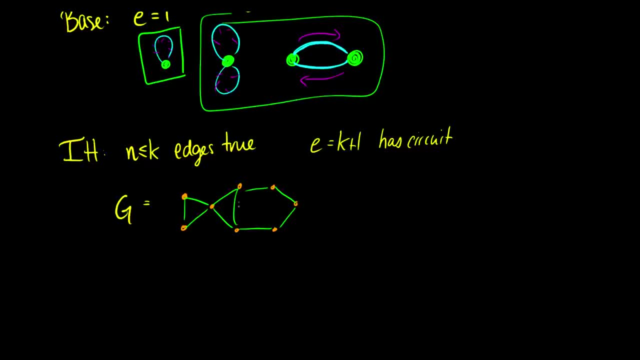 even degree. We have one problem here, So we're going to do that. Now it looks like this graph obeys everything I want it to. Okay, so it's connected and each vertex degree is even Okay. So what we're going to do next is: we're going to construct an Euler circuit Or we're not going. 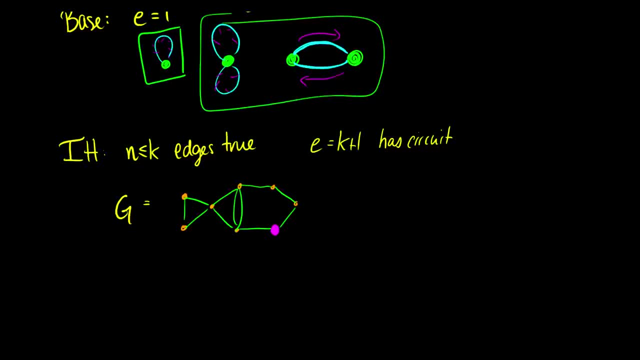 to construct an Euler circuit. We're just going to construct a circuit, So we're going to start here and we're just going to construct a circuit. So let's do that and say: okay, we go here, We go here And we're just going to go around. So there we go. That's a circuit, we're going to call that. 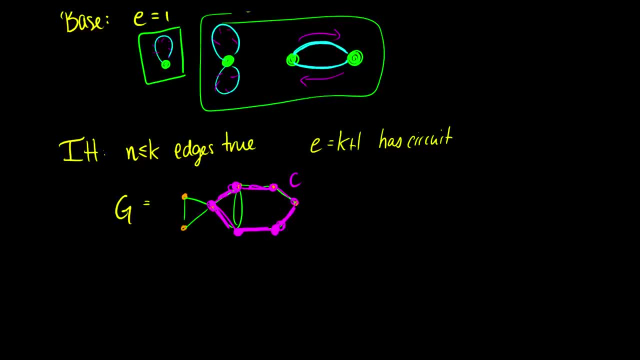 circuit C. well, it's connected and each vertex degree is even so we know there is some circuit in there. doesn't matter where the circuit is, doesn't matter how long it is, we're just gonna have a circuit. so there's two cases here. case one is that we pick a circuit that is an Euler circuit, and if that's, 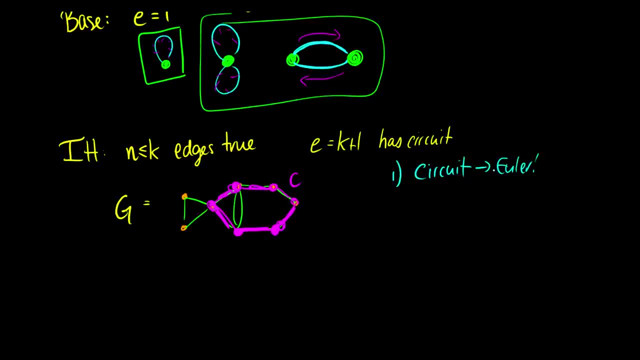 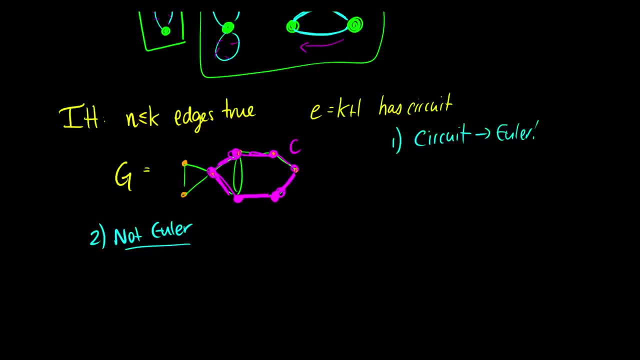 the case, then we're done, because we've proven that the graph has no other circuit. but the case that we're actually interested in is the case where you pick a circuit and it's not an Euler circuit. so what do we do then? well, we're gonna copy and paste our little graph here and we're gonna deal. 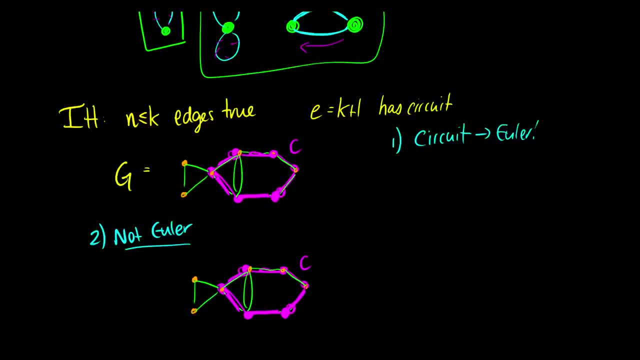 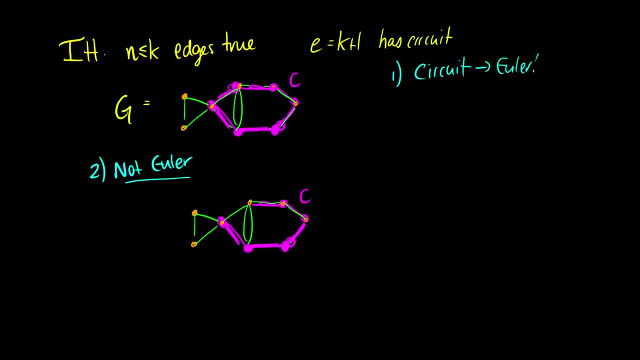 with this, okay. so what happens if we pick not an Euler circuit? here's where the fun part comes. we're going to decompose it, which means everything on our original circuit we are just going to delete. okay, so get rid of the pink there. so this is what we're left with. we deleted our original circuit, so here's the thing when we do. 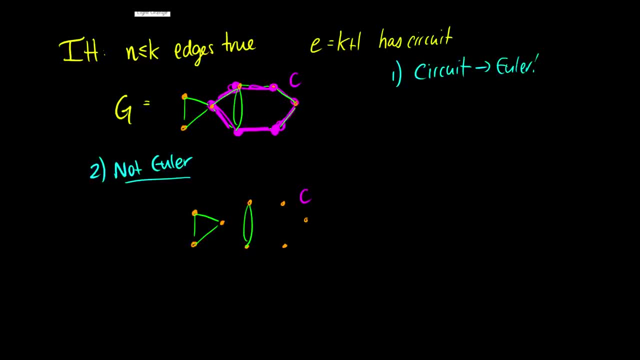 that. what do we notice about the leftover components? well, the leftover components are all Euler circuits. so there's an Euler circuit here and an Euler circuit here, and what do we know? well, it's going to be a connected graph still. it's going to be a graph with even degree vertices still. and what do we? 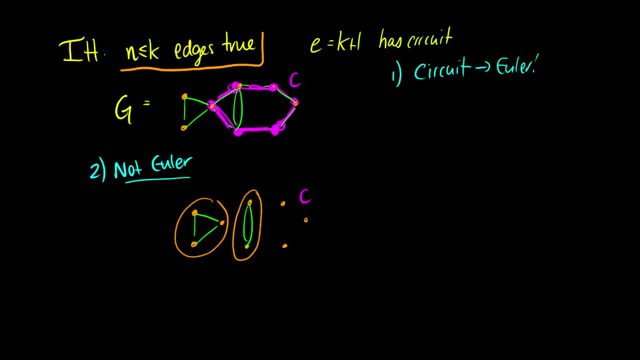 know well, we assume that if it had less than or equal to K edges, then it was true that it had an Euler circuit. so we know that whatever components remain have an Euler circuit based on our induction hypothesis. so because of our strong induction, if we make this, any graph we want, we can. the graph we're working with it can be any. 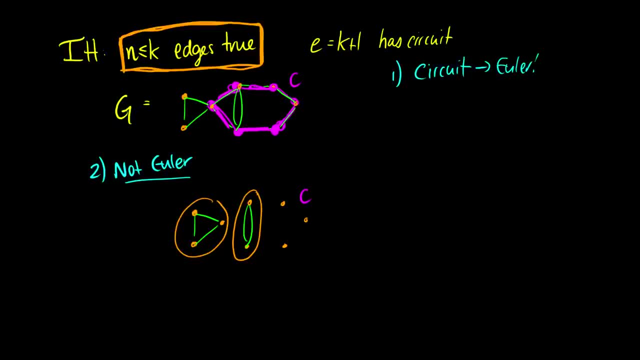 different graph. we know for sure that all the remaining components have Euler circuits, so we've decomposed it. now what do we do? well, what we're gonna do is we're gonna start back at our original position. we're gonna start back at our original position and you remember, we had our original circuit. so what we're gonna do is we're going to move along. 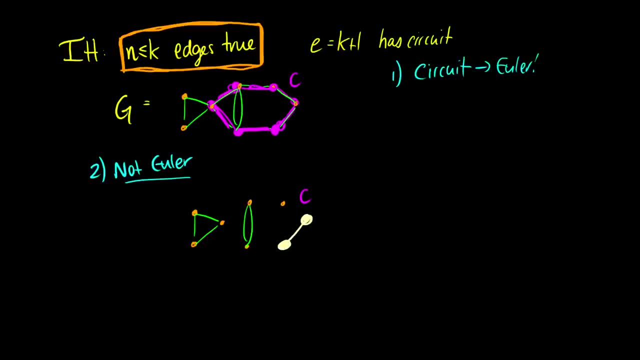 that circuit. so we get here, we get the next spot, and then whenever you touch a vertex that has an Euler circuit, we're going to take that Euler circuit. so we're going to go all the way around. so we now covered this Euler circuit and then, because this had a mini Euler circuit, we're 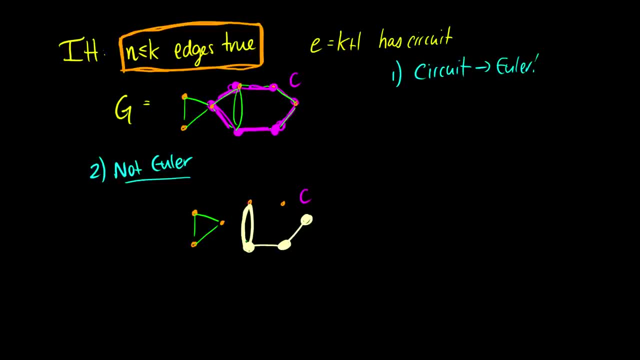 going to start and end at the same spot, so we're going to continue along the original path. and then, what do we got here? well, we hit another Euler circuit, so let's take that. okay, we're going to go through here, take it back, and now we're going to continue along. 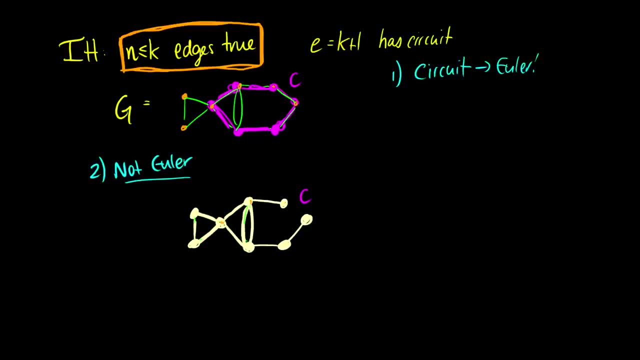 the original circuit we chose and now we have a full Euler circuit. so the proof is complete. I didn't write down too many words because I don't know why. I didn't write down too many words because I don't know why the world is so complex. it takes a lot to write a lot of words textbooks do. 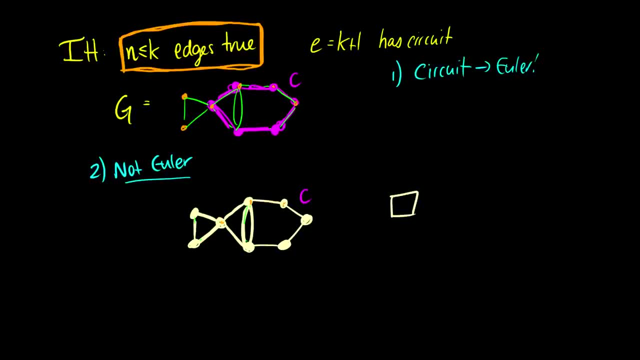 it. good, this proof is on the internet in text, so hopefully, now that you've seen visually what's going on, you can take a look at a textbook and see it in words and understand it. so let's go over this again quick. I'll do a little recap here. 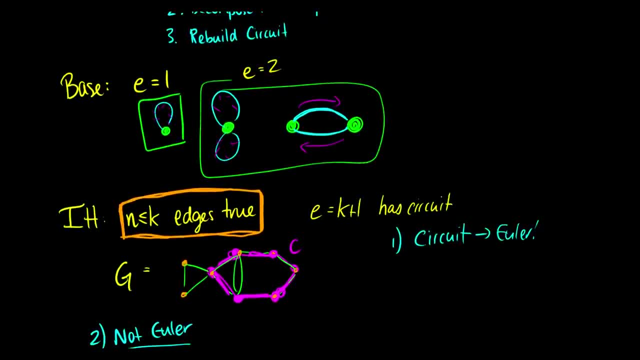 so we're going to show that if connected and even so connected and even degrees, because we want to take these two both out, and then we're going to take a look at this one and see where we went wrong. two, and we want to show there's an Euler circuit, so we assume that. so we said 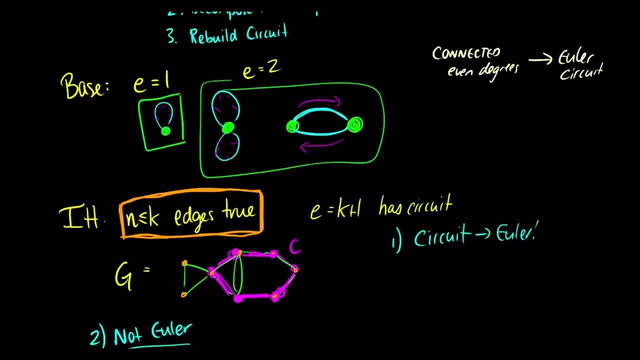 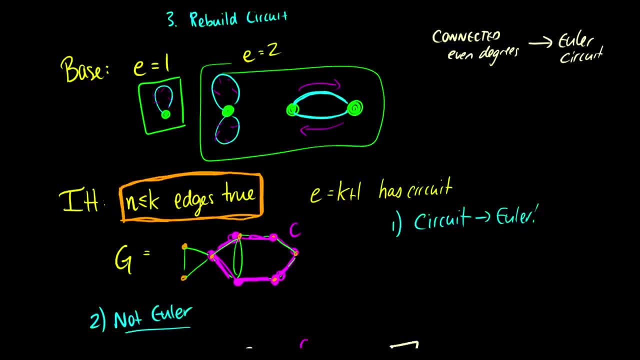 okay, if there's one edge, we can do it. if there's two edges, yes, it's gonna have another circuit for sure. so the base case is shown for the induction. we said: okay, let's, let's say all edges less than or equal to some number. K is gonna have. 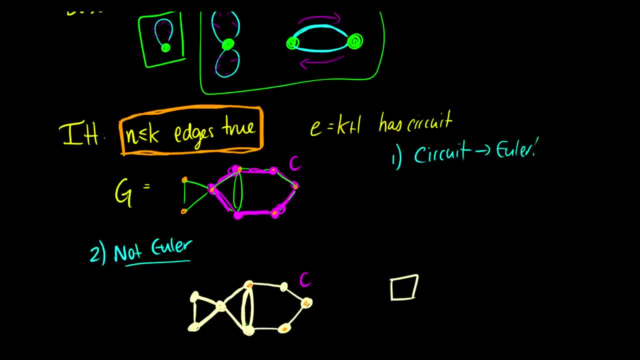 an Euler circuit. and then we're gonna say: let's go one step further and show that that has a circuit. let's add an edge. so we take any graph we want and we construct a circuit. there's two cases when we do that and I should say we know. 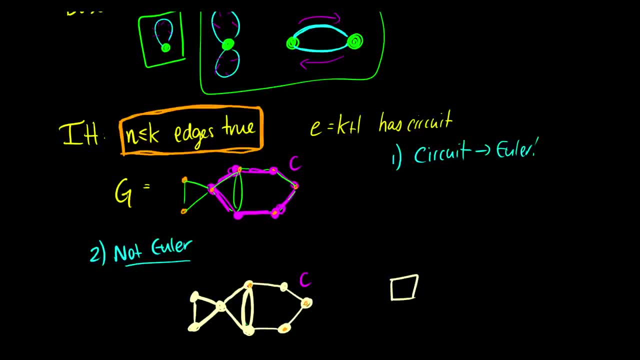 there's at least a circuit, because connected and even degrees mean that you can leave and enter every single vertex, so there must be some path to get back to the original. okay, so that's been done. if we pick a circuit, nicely, it could be an Euler circuit right away, if not. 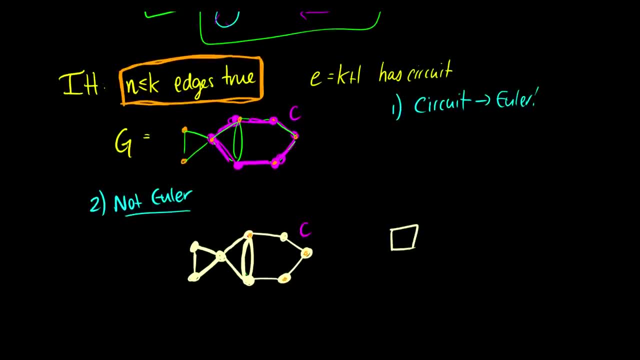 you can do it if you want to do it. if you want to do it, if you want to do it, you can do it if you want to do it, if you want to do it, if you want to do it, then what we do is we delete the original circuit, so we delete all those. 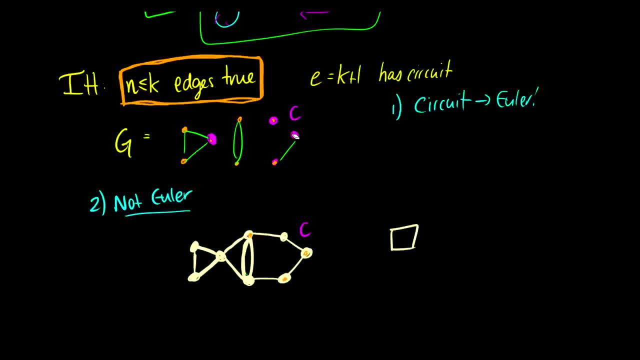 edges and we delete our little pink circles. and then what we do is we take a look at the remaining parts and because our induction hypothesis said for n, less than or equal to K, it has an Euler circuit, we know that the number of edges in our components are going to be less than. 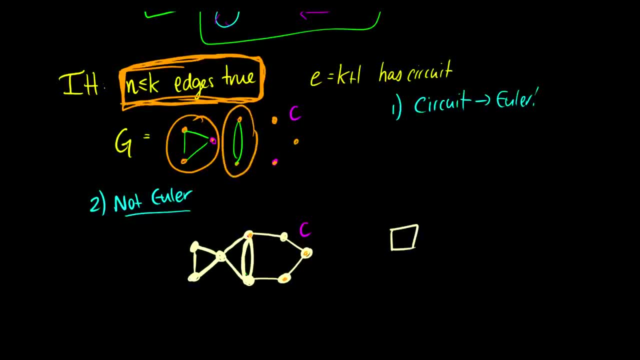 K. so that means that when we reconstruct our circuit we can just take the Euler circuits as we hit the vertex that contains them and then we construct a full Euler circuit in the graph. so that's the proof- a little complicated, definitely the first complicated graph theory proof you've probably seen. and 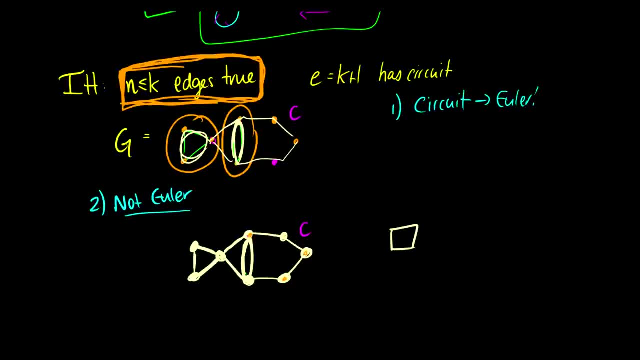 it's gonna get probably about the same difficulty for the rest. so conceptually, visually, if you can do this visually, you can figure out the words to make it work verbally or written. so hopefully you understand the main concepts behind that. so let's take a look at directed graphs. 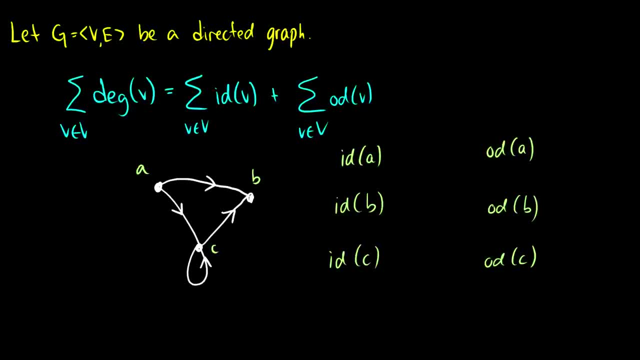 so directed graphs have a different degree structure. the total degrees in a directed graph is still two times the amount of edges, but because directed graphs have directions, which means there's heads and tails. we talk about in degree and we talk about out degree. so this is in, this is 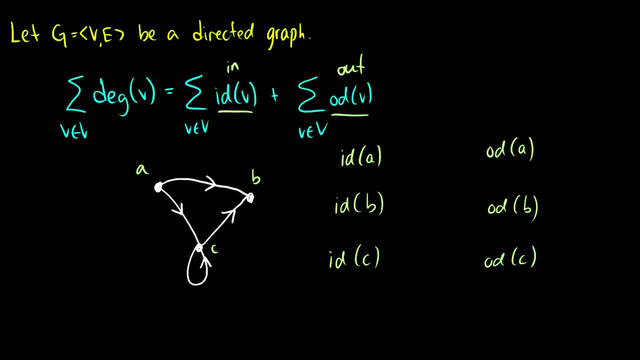 out. so an in degree is when the head points to it and an out degree is when the tail comes out of the node. so let's take a look at the in degree of a. so we take a look at a here and we say, okay, nothing's coming into it. 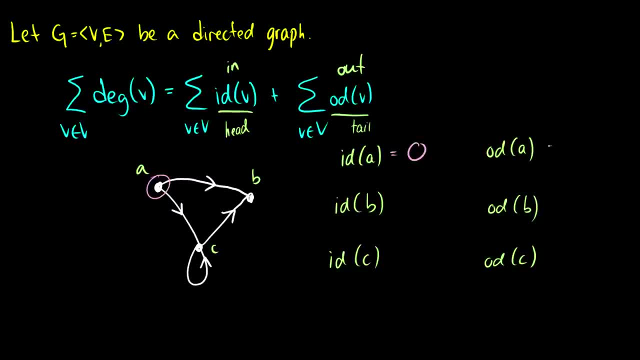 so the in degree is 0. what is the out degree? well, we have one edge going to C and one edge going to B, so the out degree is 2. okay, let's do B the in degree? well, it has nothing going out, so it has an in coming from a and an in. 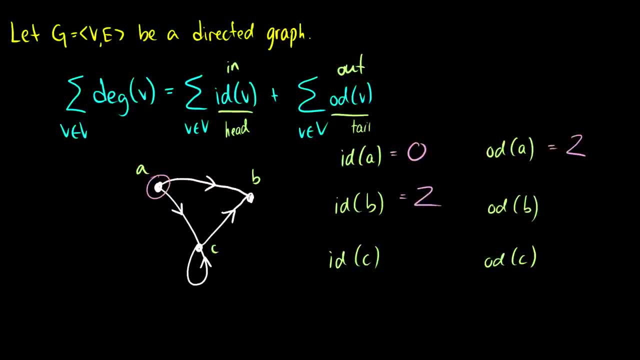 coming from C. so the in degree of B is 2 and B doesn't go out to anything, so the out degree is 0. okay, what about C? the in degree has one coming from a, but it also has one coming from itself, so that's 2, because one comes from a and one comes from itself. now the out degree. 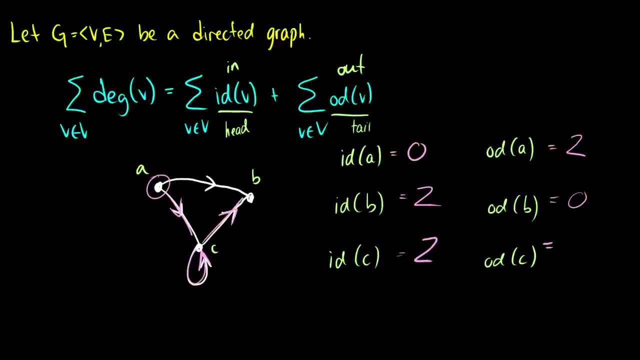 has one going to B, but it also has one going from itself to itself. so this is plus one going to B and plus one going to itself, so that's two. so when you have a loop, you have in degree plus one and you have out degree plus one. so, again, just like when you have a CC here let's take a look at how. 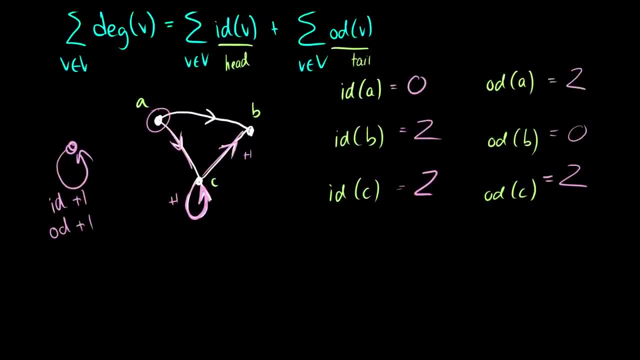 we write edges, so remember in directed graphs, when we have an edge it's ordered. so we have CC. the first position is always going to be the out degree and the second position is always going to add to the in degree. so we have CC. it adds one to the out degree for C and one to the in degree for C. so 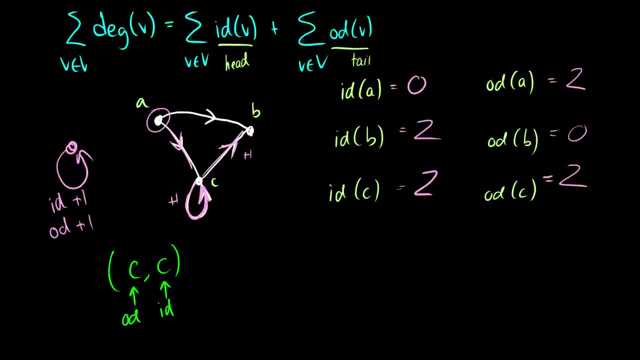 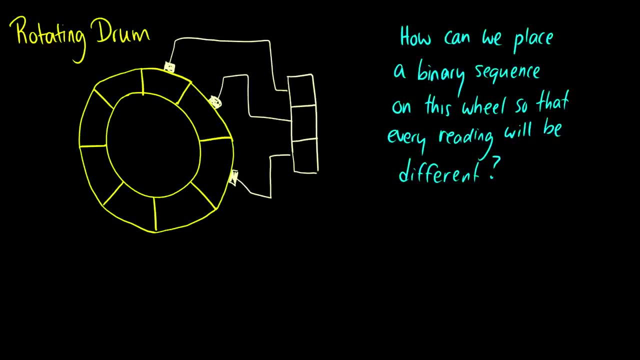 that is how we do directed graphs. so why do we need directed graphs and why do we need Euler circuits and trails? this is really complicated and I don't really see an application. well, lucky for you, there's a nice application that takes in directed graphs and Euler circuits. so that's the first position and the second. 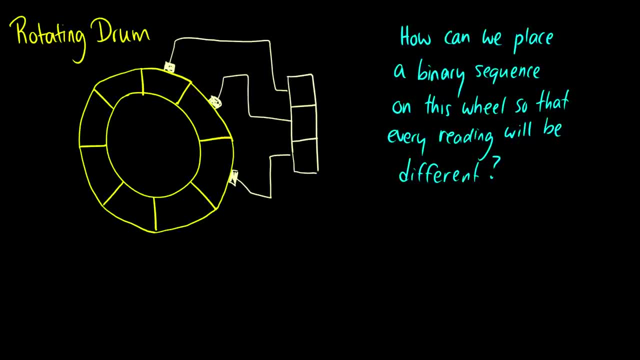 circuits. so rotating drum. here's what a rotating drum does. it connects to three different nodes here. so what we have on the right is some display. so this might say 1, 0, 1, and this corresponds to the numbers on a drum. so this drum right. 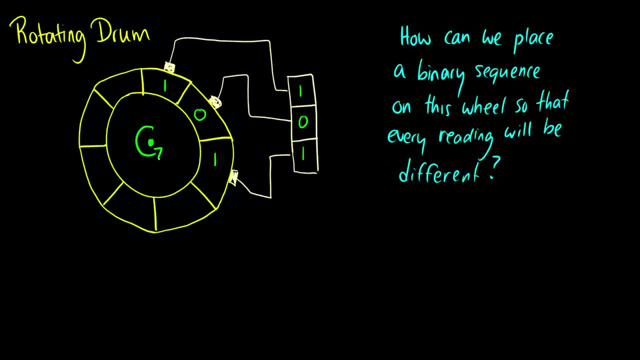 here. it's gonna rotate in water or in some electrical plant- who knows what it's for, but it's gonna rotate and based on the three inputs here, we are gonna know what position the drum is at. so let's say we're measuring strength and it has some resistance meter and when it said zero, zero, zero, it's not moving at. 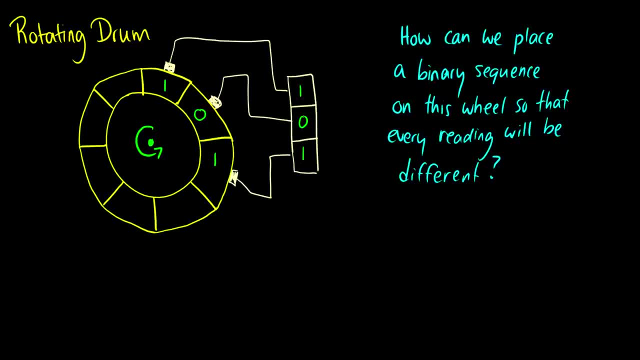 all. but when it's at 1: 1- 1 it's moving really, really hard and it turns based on how much flow we have going through. so it's a little bit hard to imagine and probably doesn't obey the laws of physics, but it could measure strength. so what we want is we 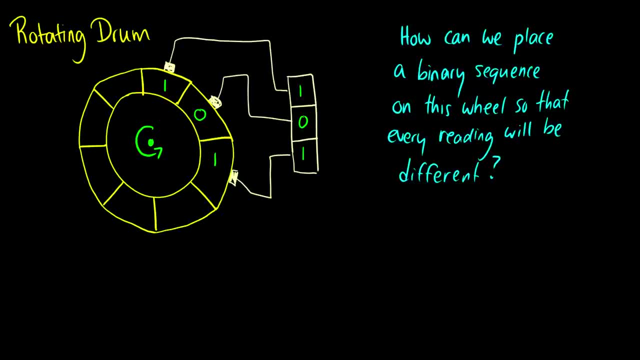 want to put down a binary sequence of digits so that no reading is exactly the same, because let's say, we have 1 0 1, 1 here. if this all moves over one position and then the new reading is going to be 0 1 1, so this will get replaced with 0 1 1. so 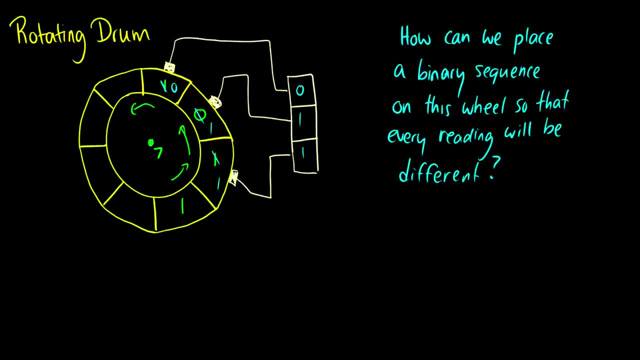 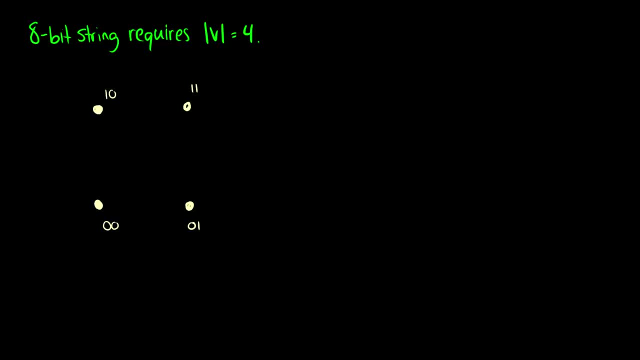 we want all of these different readings to be different when we rotate it. so how can we figure out a nice sequence to put on this drum? well, we're going to use an Euler circuit, so an 8-bit string is we're going to require that we have four. 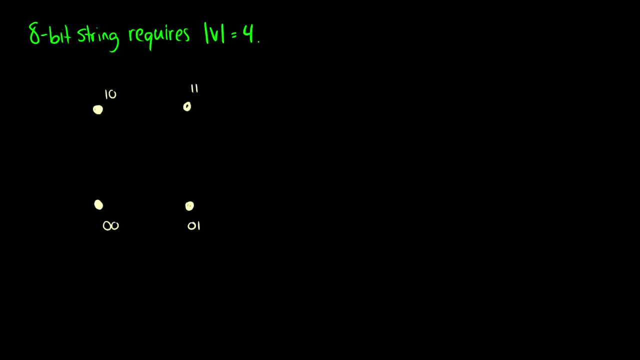 vertices. a 16-bit string would require eight vertices. so when you double the string, you double the vertices. so let's take a look at how we construct this. so we're gonna do this with a graph. and how do we construct the graph? well, what we do is: 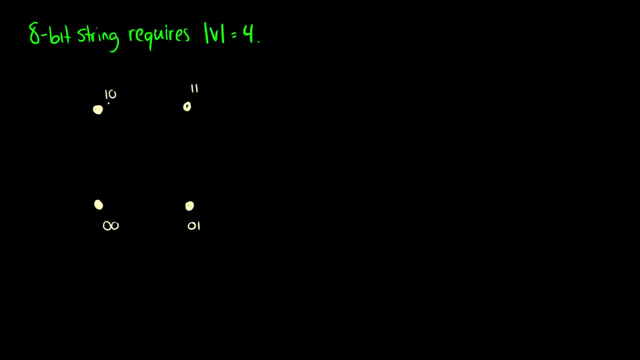 we take this 1: 0 here. we're gonna start with 1: 0 and let's say we have a node 1: 0 when we connect it to something. we're gonna take three digits. the first digit is going to be the 1, 2nd it's going to be the zero and the third digit is going 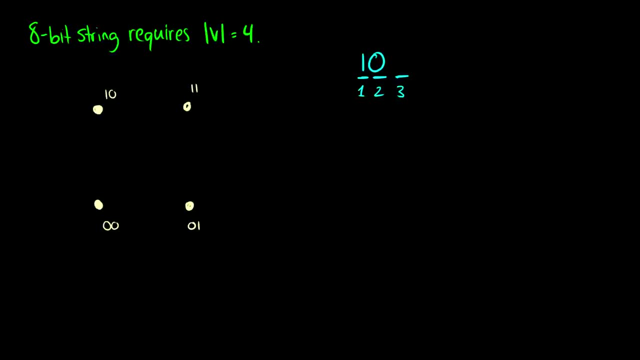 be the vertex that we point to. But what's going to happen here is when we take a look at, say, another node, let's take a look at 1, 1.. Let's say we're going to 1, 1.. The first digit is going to. 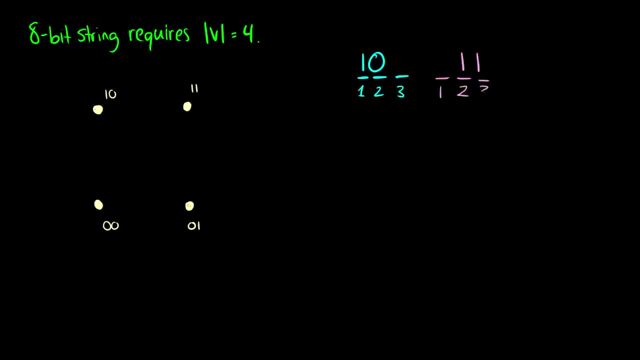 be a known. the second digit is going to be 1, and the third digit is going to be 3.. So the node that we come from is going to have the first two numbers and the node that we go to is going to 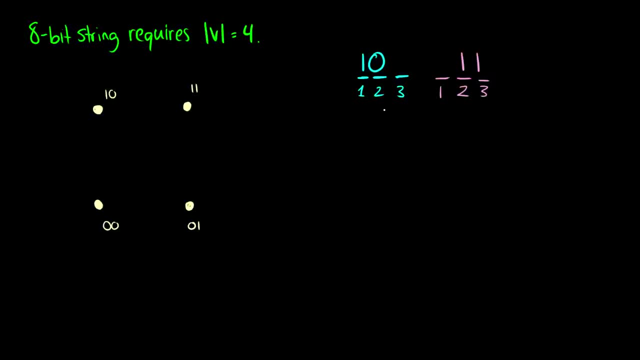 have the last two numbers, which means that these two positions here have to be the same number. So, as an example, this 1, 0 can go to 0, 0.. Let's just do this. So 1, 0 can go to 0, 0.. So we get a. 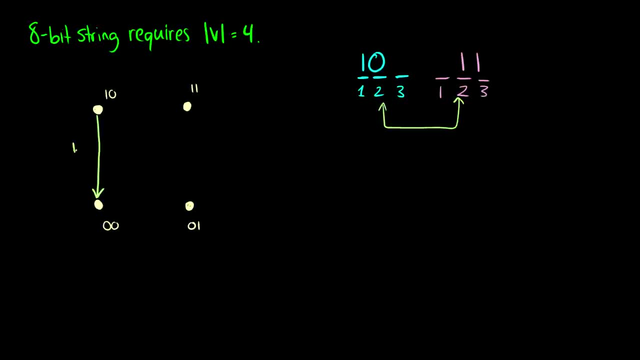 1, 0.. Let's do this on the outside. here We get a 1, 0 from the first node and then we go to 0, 0, which gives us the second and third numbers. So this edge is going to be 1, 0, 0.. 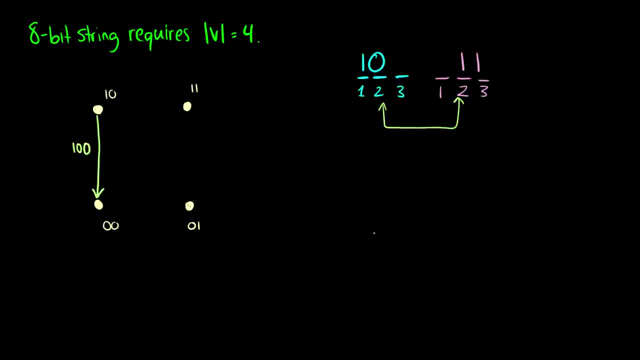 So, just to show this, we have three positions. We come from 1, 0.. We go to 0, 0, and this is all going to collapse to give us 1, 0, 0.. Let's do another example here. We're going to go from 1,. 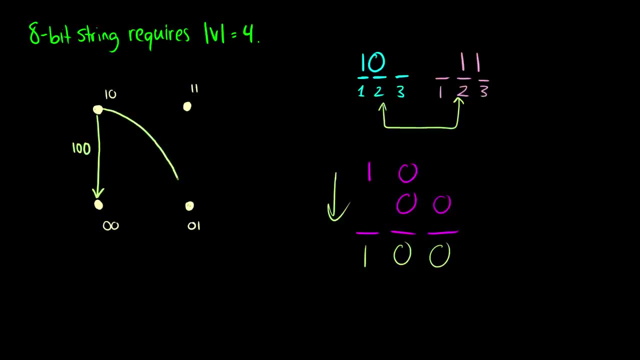 0 to 0, 1.. So we're going to get 1, 0, 1.. So let's see how this works. We take the 1, 0 from the first number and the 0, 1 from the second number or the second vertex. 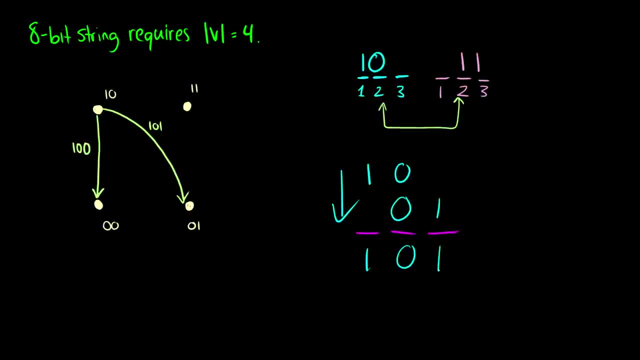 and this collapses down to 1, 0, 1.. Okay, so let's just fill out the rest here. We're going to do this for all the possible values, So we can go from 0, 0 to itself and get. 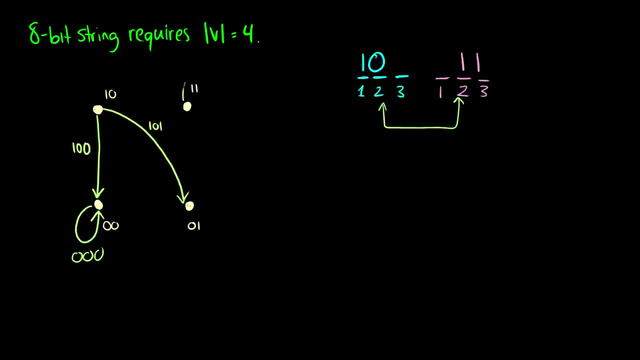 0, 0, 0.. Go from 1, 1 to itself and get 1, 1, 1.. 0, 1 can go back to 1, 0 and we'll get 0, 1, 0.. 0, 0 goes to 0, 1 to give us 0, 0, 1.. 0, 1 goes to 1,. 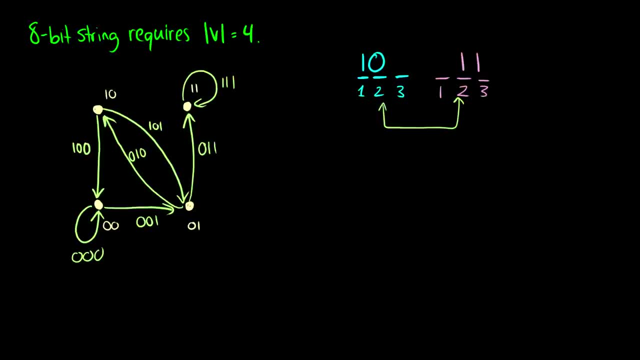 1 to give us 0, 1, 1.. And 1, 1 goes to 1, 0, to give us 1, 1, 0. So you can do that example for all of these As mentioned. these have to be the same, so you can. 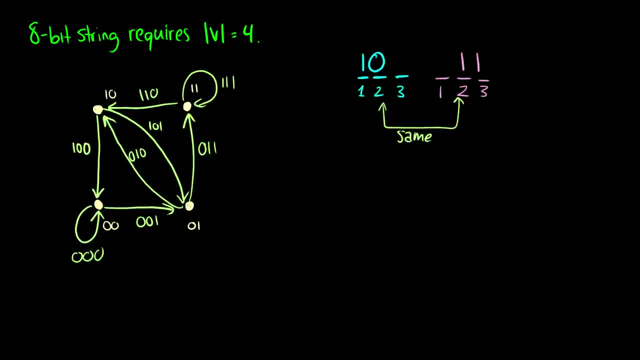 test each one individually to collapse it, But this is the resulting graph we get. Now we're going to type in a new arrangement to create a new시- shame. So we're going to do this by opening the code, Because this should go like this in the last� 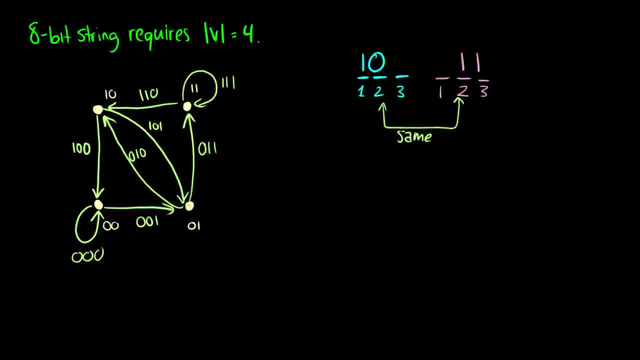 we'll do is we need to make a sequence somehow. So what we're going to do is we're going to construct an Euler circuit So we can start wherever. Let's start at 0, 0. Then what we'll do is we're just going to draw as we go. So we're going to go from 0, 0.. We're going to take this. 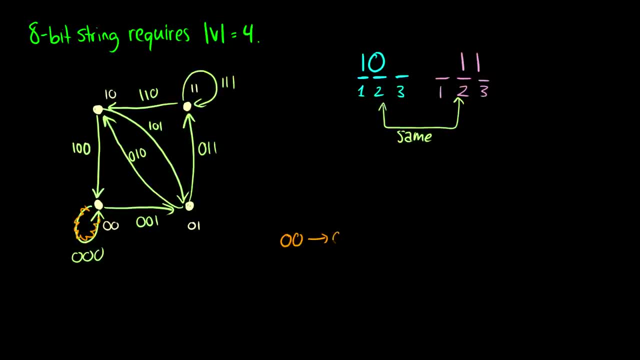 edge right here and go back to 0, 0. Then we're going to go. well, we can only go to 0, 1 right now. So let's take this edge and go to 0, 1.. Now, with 0, 1, let's go up to 1, 0. Then we can go. 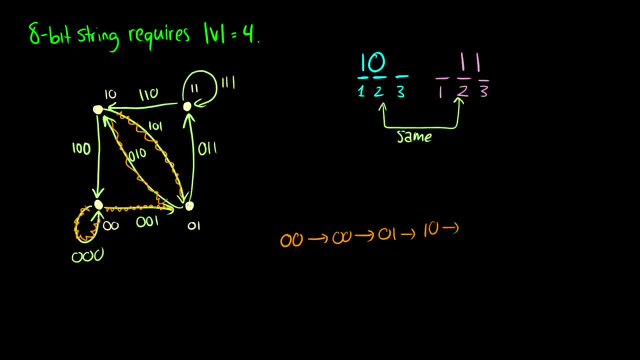 back down to 0, 1.. Then let's go all the way up to 1, 1.. Just keep following the edges, one by one. Then we'll take 1, 1.. We'll loop it back around to 1, 1.. Then the only place we can go now is 1, 0.. 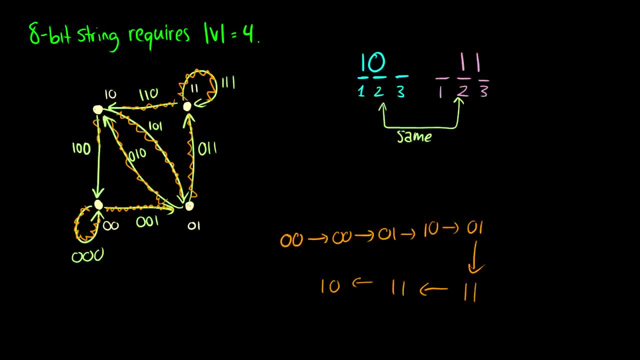 And then we have to loop back to 0, 0. And that ends the circuit. Okay, so we need an 8-bit string. Well, let's take a look at this. We have 1,, 2,, 3,, 4,, 5,, 6,, 7, 8 vertices in our circuit. 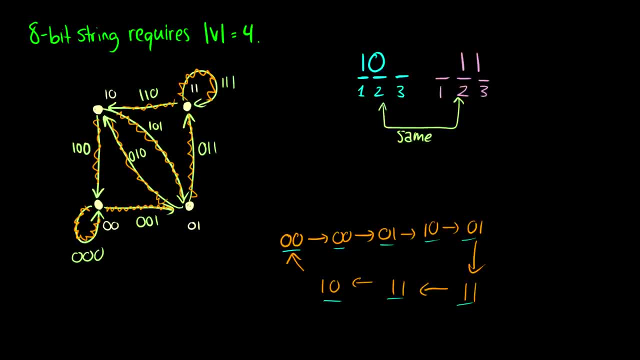 So what should we do? Well, we take the first number from each of our vertices And then we just make a list of those numbers And we follow the Euler trail. So we're going to get 0, 0,, 0,, 1,, 0,, 1,, 1,, 1.. And this is going to be our binary sequence. that fits into the drum.